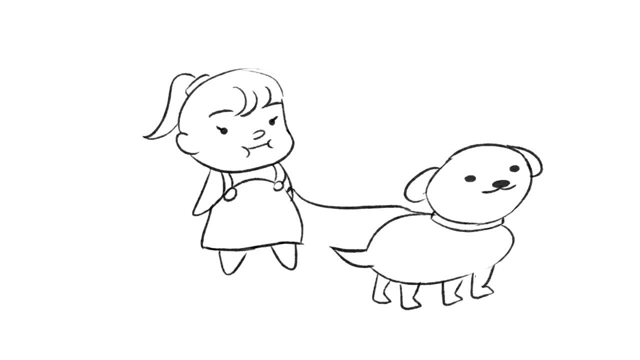 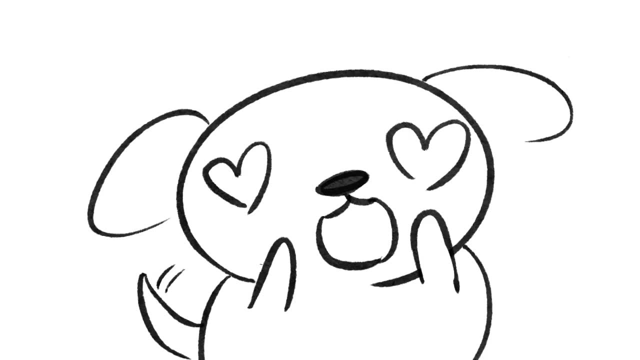 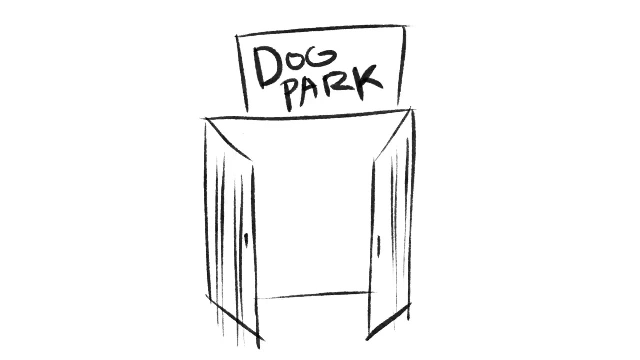 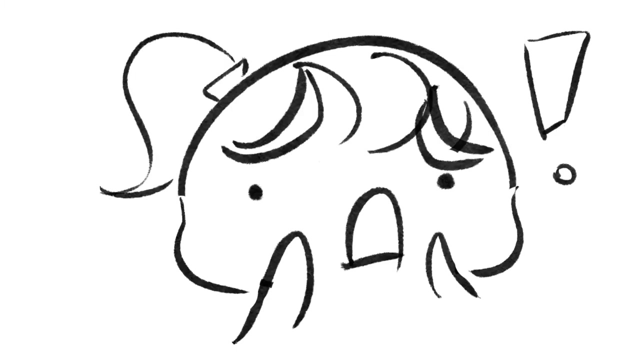 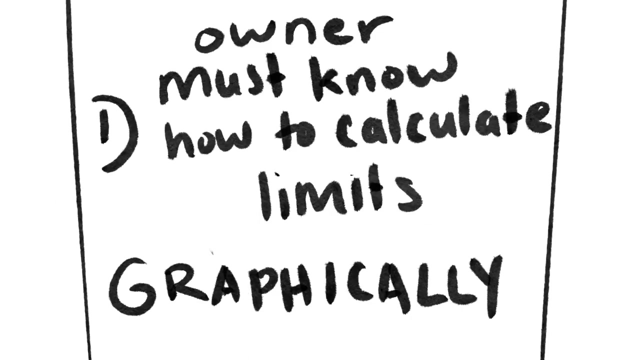 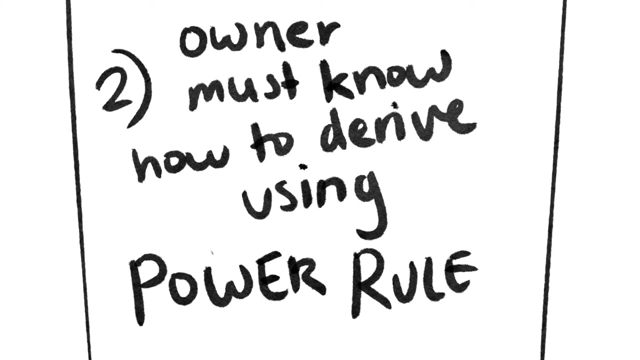 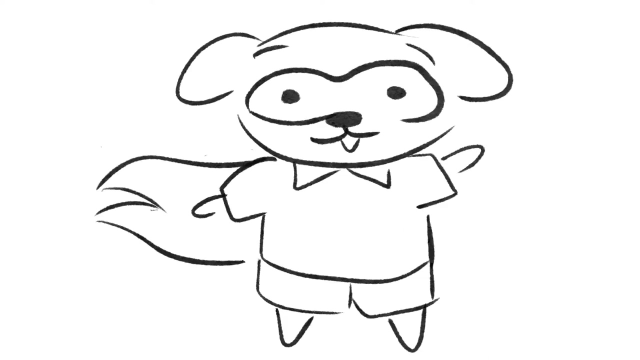 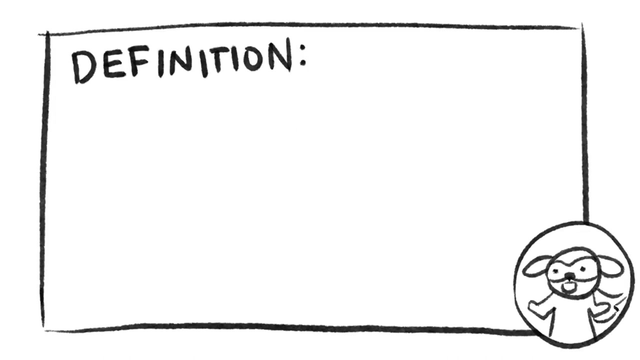 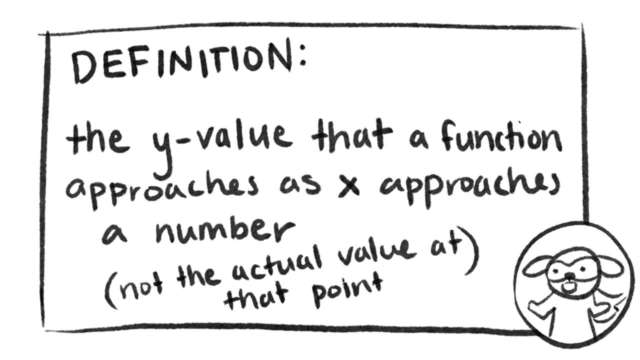 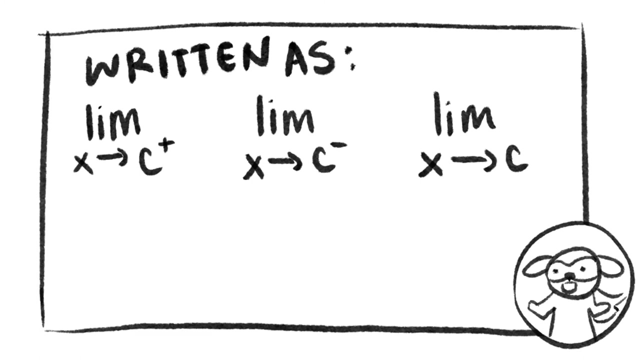 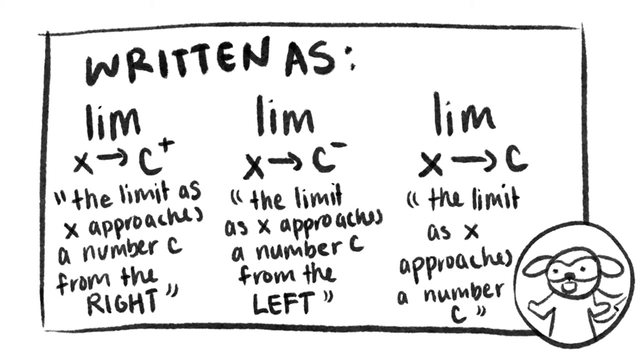 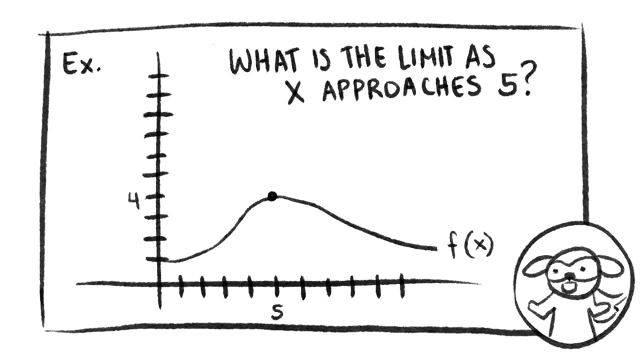 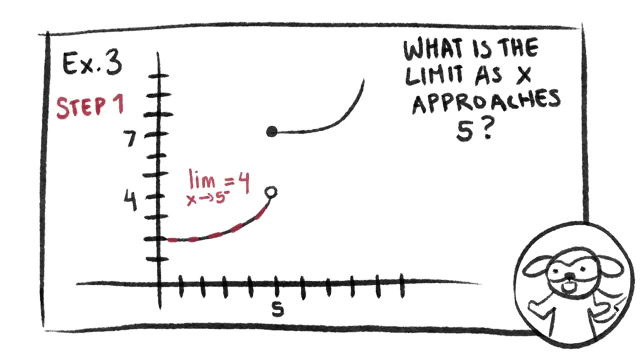 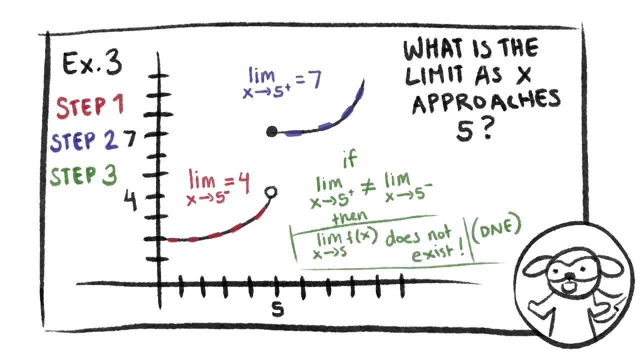 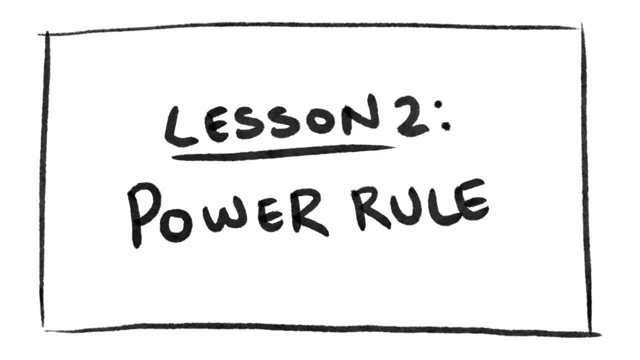 then the limit as x approaches 5 does not exist, or DNE for short. Good job. Let's move on to the next lesson, Lesson 2.. Power Rule. We have two functions, 2x and 5x, cubed. 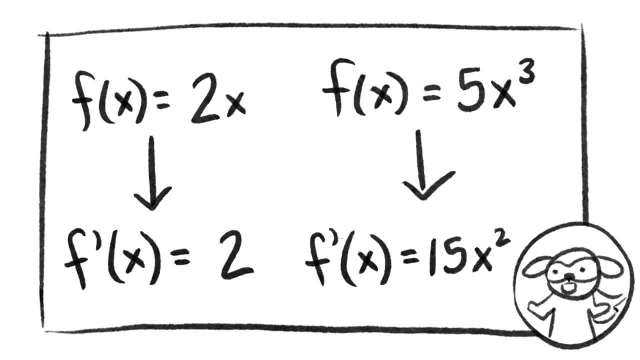 When we take the first derivative of 2x, it will equal 2.. For 5x cubed it will equal 15x squared. How did we get the u-ask? We use the power rule. It's super easy.